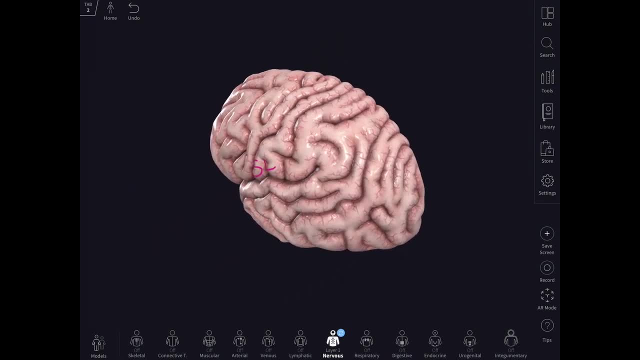 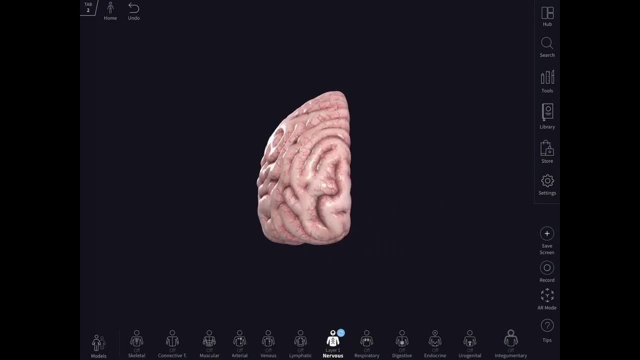 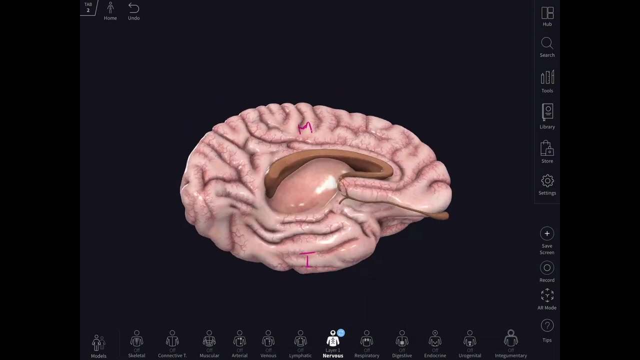 So the surfaces are: you have a convex, a supralateral surface, So this is a supralateral surface which is convex. Then you have a flattened medial surface, So this is a medial surface which is flattened. Then you have a irregular inferior surface. 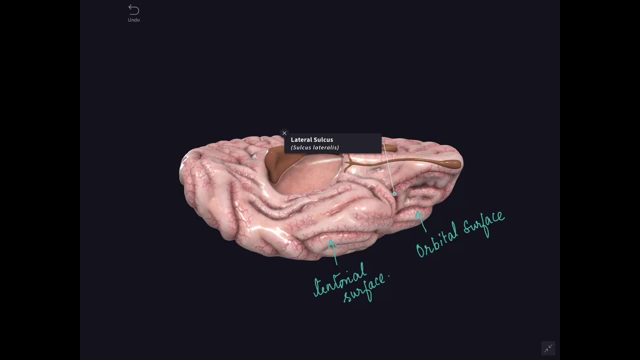 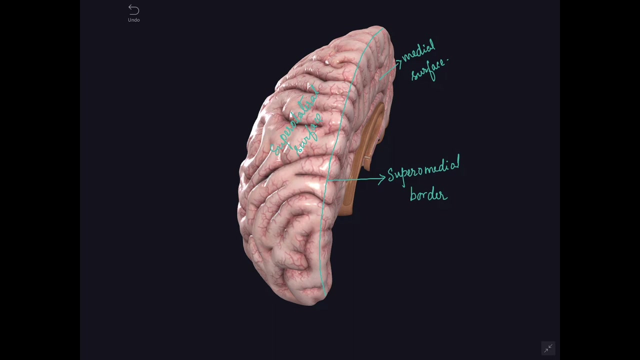 The inferior surface is further subdivided by the stem of the lateral sulcus into an orbital surface in front and tentorial surface behind. Next we will see the borders. So first we will see the supramedial border. The supramedial border lies in between the supralateral surface and the medial surface. 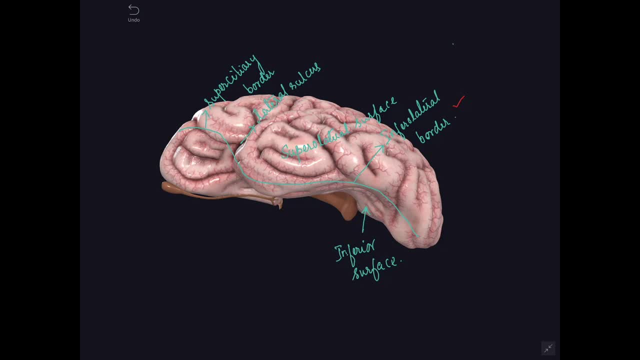 Next we will see about the infralateral border. The infralateral border separates the supralateral surface and the inferior surface. The part of the infralateral border in front of the lateral sulcus is known as the supraseal border. 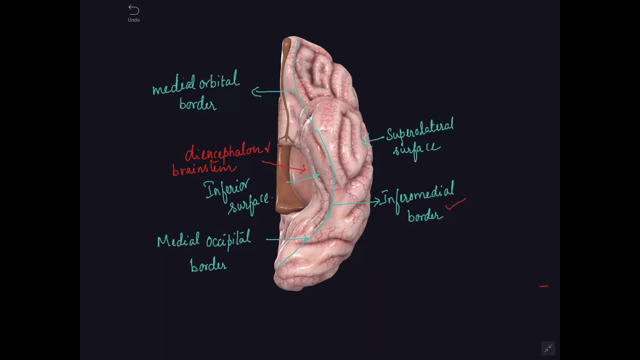 Now we will see the infromedial border. The infromedial border separates the supralateral surface from the inferior surface, So this border is interrupted by the diencephalon and the brain, stem into a medial orbital border in front and a posterior medial occipital border. 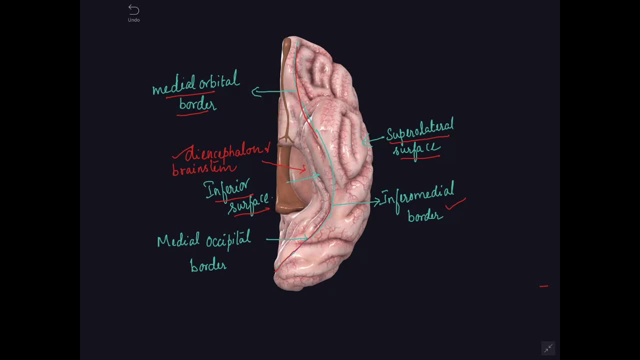 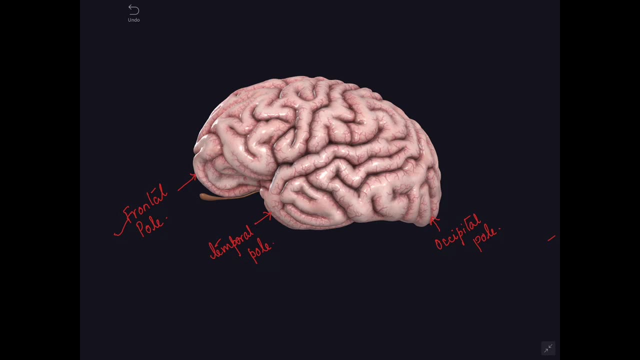 So what we will see is that we have a lateral sulcus And this lateral sulcus is a medial oxipital border And this lateral sulcus is a medial occipital border. Now we will see the poles. We have a frontal pole in front, an occipital pole behind and a temporal pole below and in front. 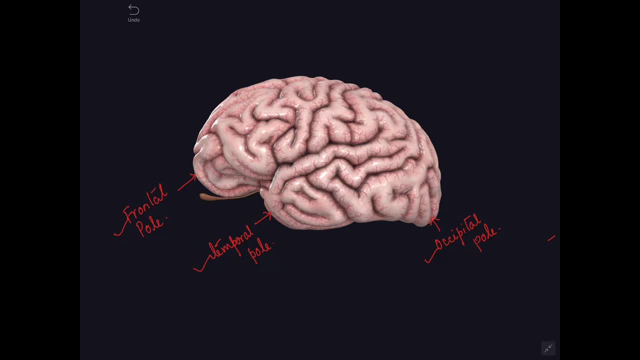 The temporal pole is the primitive posterior pole which is curved anteroinferiorly for better accommodation. The frontal pole is supplied by the cortical branches of the anterior cerebral artery, The temporal pole is supplied by the middle cerebral artery and the occipital pole is supplied by the posterior cerebral artery.